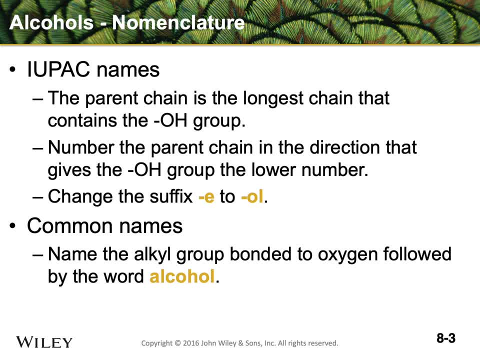 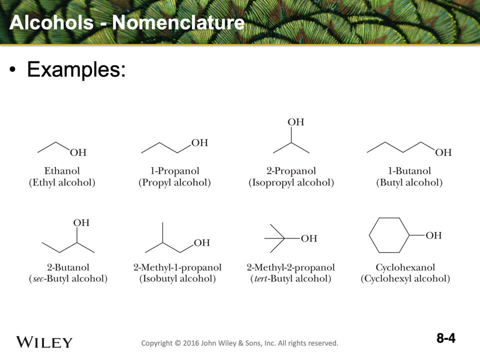 that's bonded to the oxygen and follow it by the word alcohol. Let's do some of those for an example next. So in this case, right here we have ethane right here, but we have now the OH on the end, And so we cut off the E and add OL to give us ethanol. Here we have one, two, three carbons. 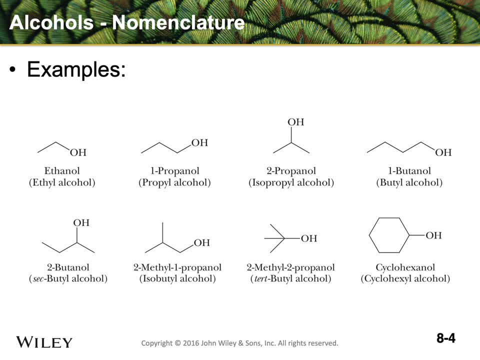 So we have propane, cut off the E, add OL, So we have propanol Right here we notice we have it on this first carbon here. So we denote that it's on the one position or the one carbon here, giving us one propanol If we were to move this oxygen over one position. 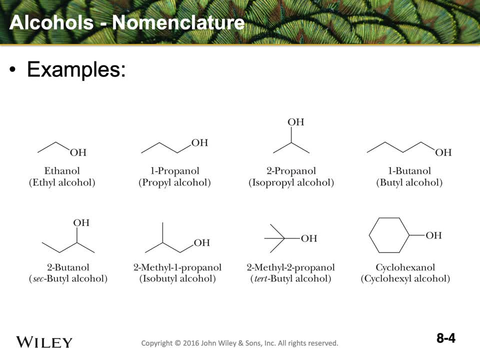 so it's on the two carbon, as in this one. we have to denote that as the two propane. When we go to something longer like butanol, right here we again have the OH on this first carbon. So we give it one butanol. If we move that OH over one position, we have to denote. 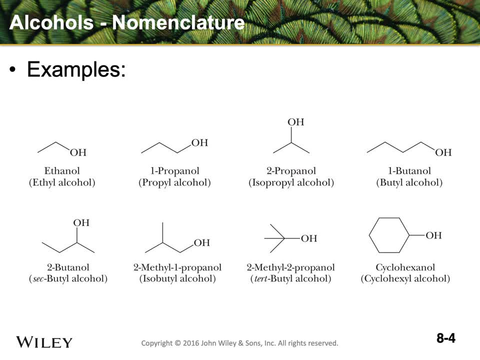 it with a number two, giving us two butanol And so, and then, as we move to higher and higher, we have to just show where that is Now, because the OH is the parent chain. we can then start naming it. 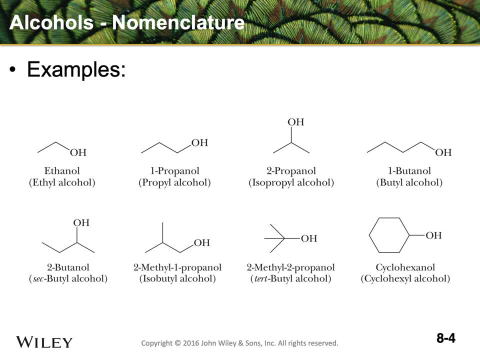 Numbering substituents from that position. So in this case, we have one, two, three carbons right here, meaning that our longest chain is now propane. So now that we have the OH on there, that takes this number one position and gives us one propanol, Now we have to. 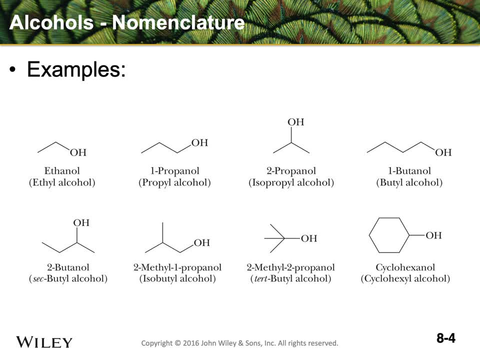 do all of our substituents from there, giving this our two methyl group. So it's two methyl, one propanol. In this case, here we again have the longest chain: is the propane, one butanol, Number two, two, three, And we have a methyl group and the OH, both on this, two carbon. 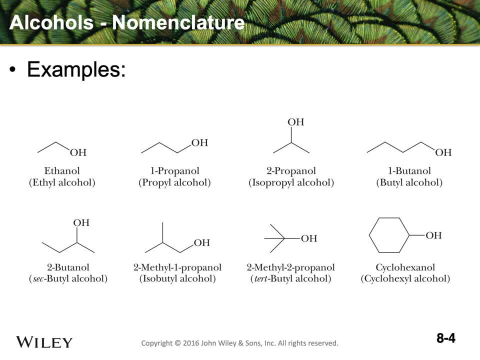 So, because the OH is on the two carbon, we have a two propanol and we have this methyl group on the two carbons. So we have the two methyl, two propanol. As with other cyclic systems, the cycle takes precedent here. So we have a cyclohexane Because we have the 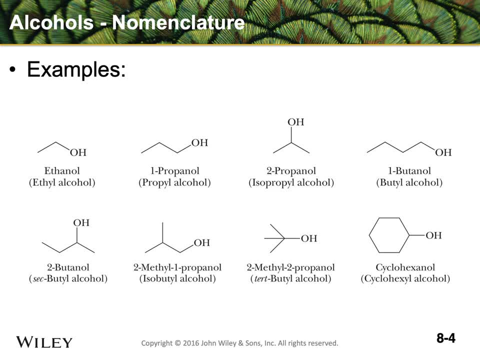 alcohol, we drop the E and add the OL to give us cyclohexanol. Now let's talk a little bit about the common names Here we have what we would call an ethyl group here. So because the common name is the group, 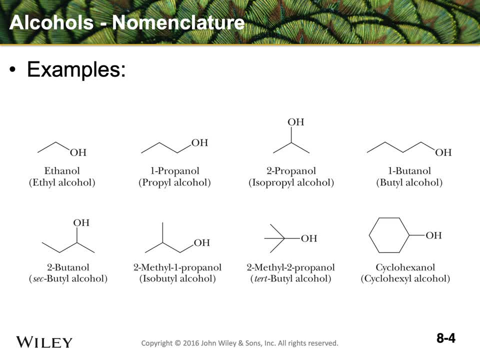 plus alcohol. we have ethyl alcohol. Here we would have the propyl group one, two, three. so we've got propyl alcohol. Now remember when we have a propyl group but something is not bonded to the end, but bonded. 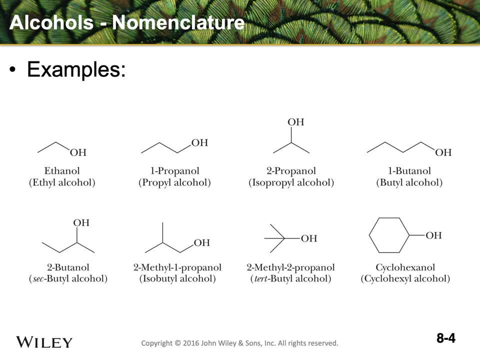 to the middle. here we call that the isopropyl group. So we end up with isopropyl alcohol. So we have our normal butyl alcohol. but then, remember, when we have our butyl group but something is bonded to the second carbon, here we call it sec or sec butyl. so in that case this: 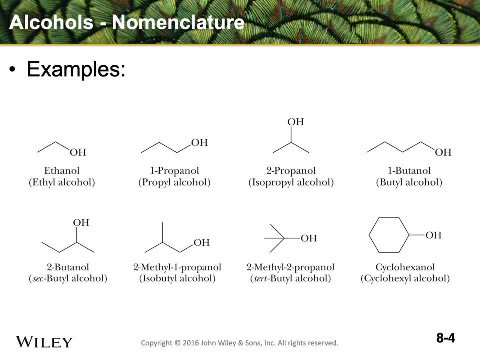 sec butyl group is now named as an alcohol, so we have the full name of sec butyl alcohol. this group right here is known as the isobutyl group, so we have isobutyl alcohol and of course the t-butyl group, or t gives us t-butyl alcohol and in this case the cyclohexyl is our substituent. 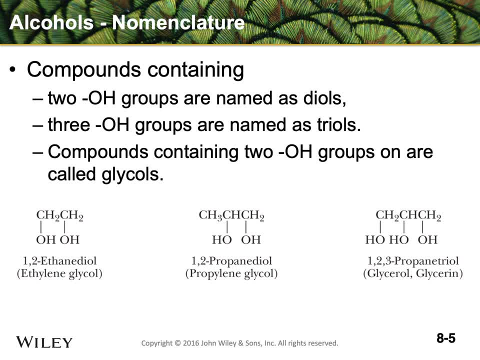 so we have cyclohexyl alcohol- okay. so we can also have compounds that have more than one oh on them, and when we have that we can call them diols. so if we have two, they're called diols, if we have three, they're called trials, four, tetraols, etc. etc. so when we name those, we name them for. 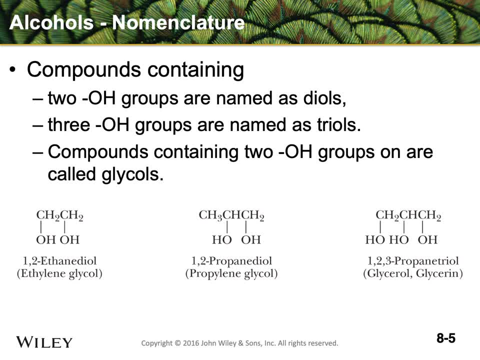 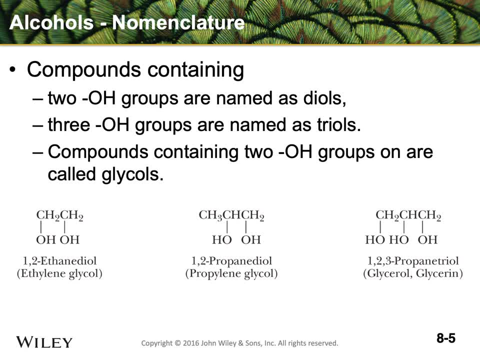 1,2-ethanediol. Here we have 1,2 position, so we have 1,2-propanediol And here we have 1,2,3-propanetriol. Now, these also have common names and they're typically. 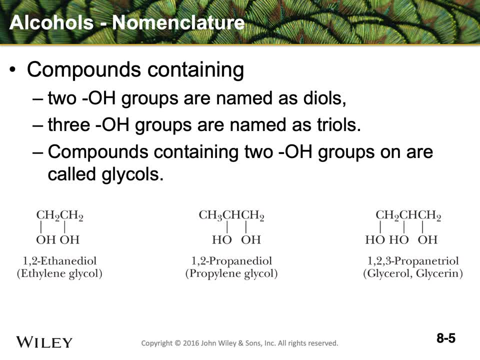 called glycols if you have two groups on there. So in this case we have just the ethyl group, so we can call that the substituent ethylene. So we have ethylene glycol Here we would have. this is propylene propylene glycol In this case. 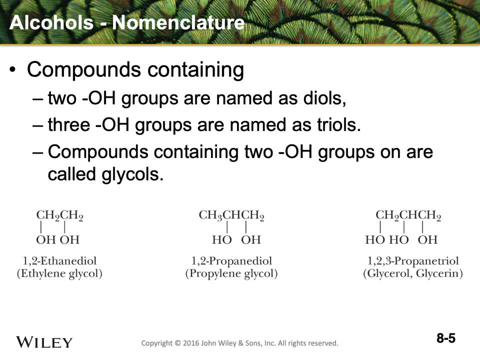 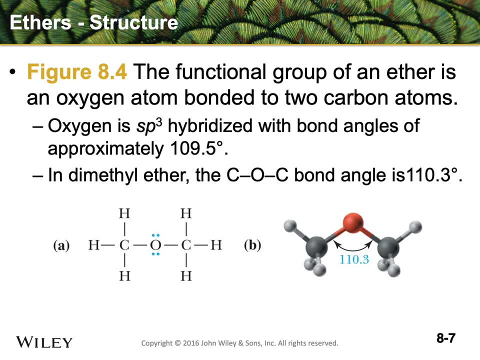 the common name is glycerol or glycer. So now to switch gears slightly: for an alcohol we have a carbon-oxygen-hydrogen bond system. In an ether we have a carbon-oxygen-carbon bond. Now the oxygen is still sp3 hybridized, which 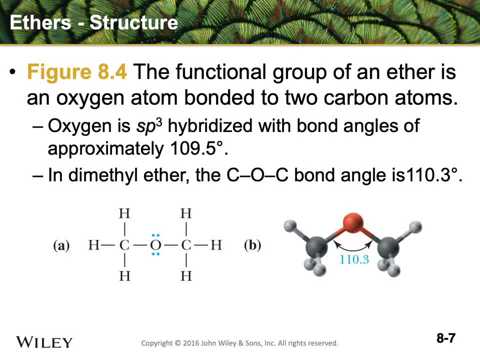 means it tries to get that 109.5 degree angle. So in all of these systems we'll see those two lone pairs there will bind together to form a carbon-oxygen-hydrogen bond. So in all of these systems we'll see those two lone pairs there will bind. 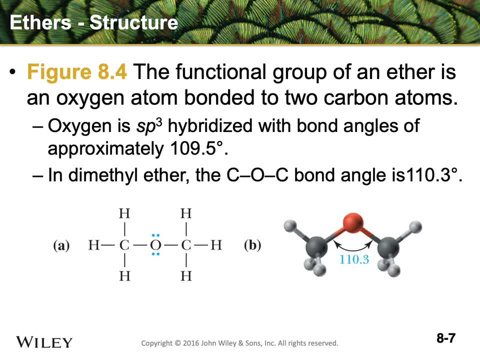 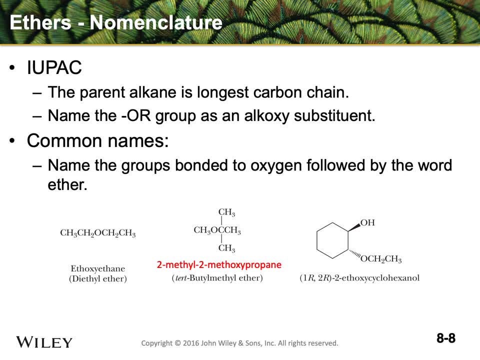 together to form a carbon-oxygen-hydrogen bond. So in all of these systems we'll see those two lone pairs. there will bind. give us a vent molecule here. electronically we are tetrahedral, Okay. so in the naming of ethers we take the parent. alkane is the longest carbon. 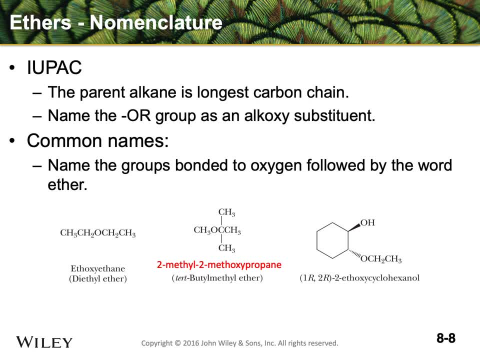 chain and then the substituent is the alkoxy group as the substituent. So in this case, here we have two ethyl groups, so one of them is going to be the parent, which is our longest chain, and then the other one is going to be listed. 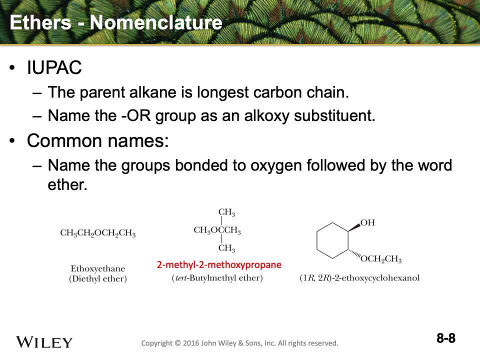 as an as the alkoxy group. In this case it's ethane, so the alkoxy group turns into ethoxy ethane, So our UPAC name is ethoxy ethane In this case. here we have one, two, three carbons is our longest chain. We have a methyl group on 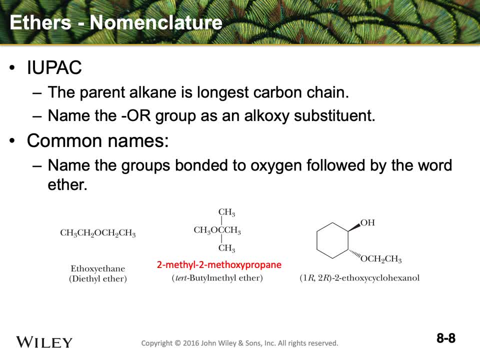 that two carbon and we have a methoxy group on that two carbon. So our final name is 2-methyl-2-methoxy-propane. In the case of our last system here, this cyclohexanol is our parent right here, because it's the 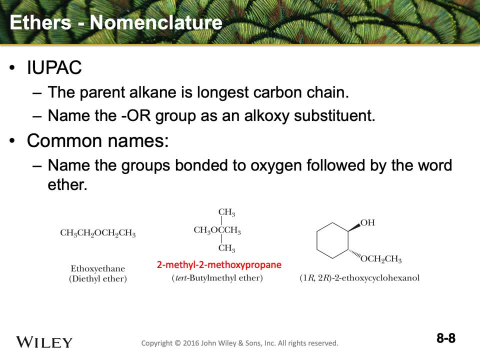 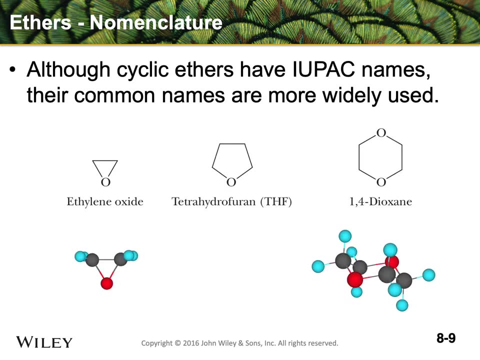 longest carbon chain, and this alkoxy group is our substituent, so we're naming it 2-alkoxy-cyclohexanol. and then, of course, we have to correctly assign our RMSs on the two stereocenters. When we name ethers, we 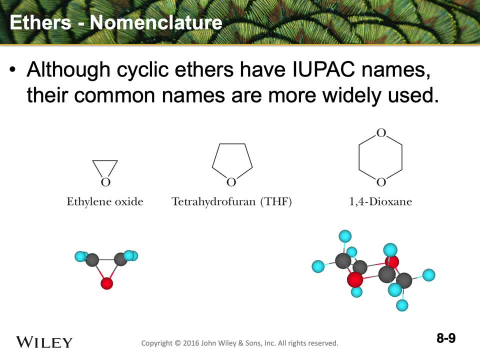 also have cyclic ethers to worry about. For example, in the case of this is our smallest cyclic ether- we have two carbons, which is ethylene, and therefore we call it ethylene oxide. Another common ether is this compound right here, which is tetrahydrofuran. We have a heterocycle here. if these were double. 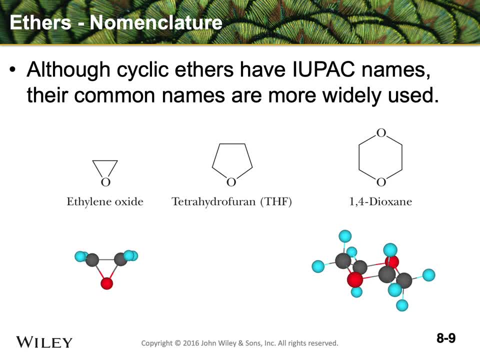 bonds. that would be called 3-uran, and so, because we're adding four hydrogens across there, we have tetrahydrofuran In this case. here we have a another heterocycle, or a cycle made up of more than just carbon, where we'd have a unit here. this is the one position, so we have one, two. 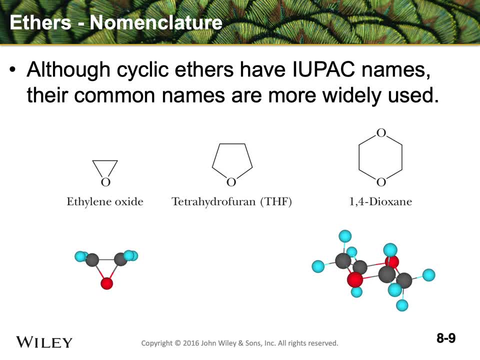 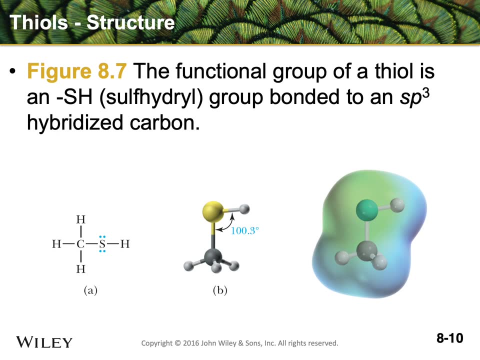 three, four dioxyalkane, so it's one, four dioxane, and so we can also have the one three position if we have the position here. The last group we're going to talk about is the functional group called the thiol, which is with a sulfur and 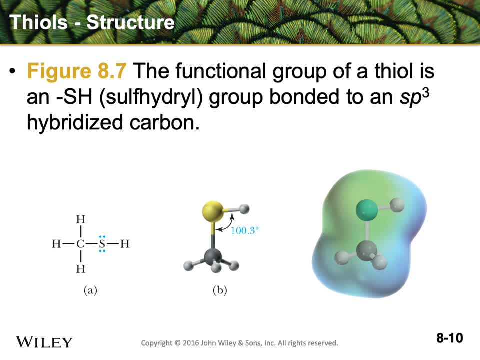 hydrogen group bonded to an sp3 hydrogenized carbon. Just like with the alcohol system, we have lone pairs on the sulfur with a hydrogen on that sulfur. Because the sulfur is sp3 hybridized, it does have that 109.5 degree bin or in. 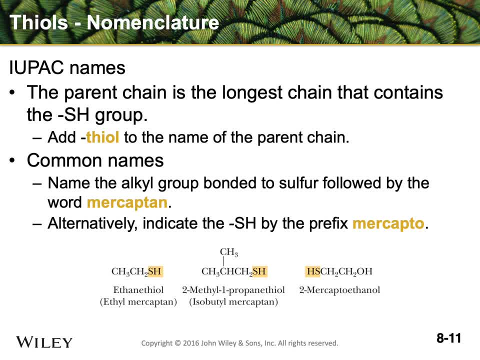 this case a little less than that. When we name thiols, we take the parent chain, the longest carbon chain that the SH group is on, and then we add thiol to the name of that parent name. For common names, we actually use the word mercaptan as a group such as methylmercaptan or ethylmercaptan. 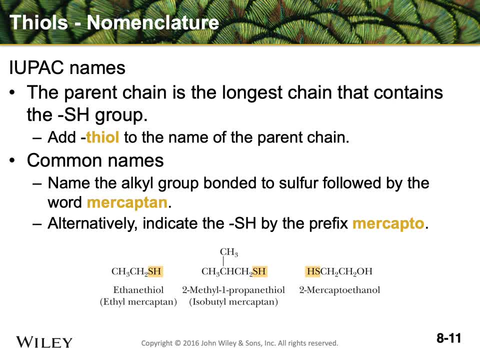 Alternatively, if you have the SH as a substituent on otherwise already named parent compound, you have the prefix mercapto. So let's look at the compounds. at the bottom here We have an ethyl group, and so we have ethane, thiol or in. 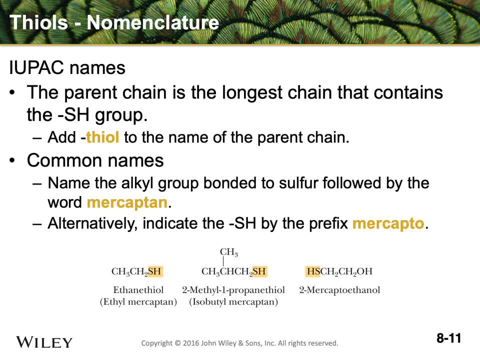 common names. we have the ethylmercaptan In the next system. here the longest carbon chain is propane and therefore we have a thiol group at the end. but we also have a substituent of methyl group, and that's on the number 2. 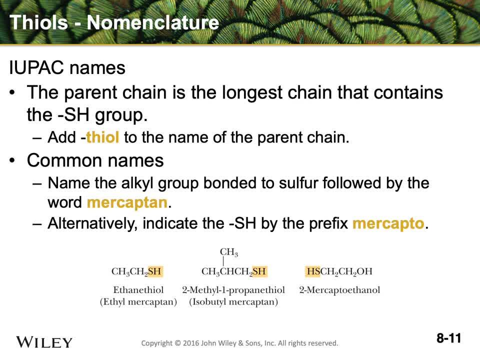 carbon, so we call it 2-methyl-1-propane-thiol. Now, in the case of the last one, here the alcohol takes precedent and therefore it is the parent chain of ethanol, and therefore we give the SH group the designation as a substituent and we call it 2-methyl-1-propane-thiol. mercapto-ethanol.